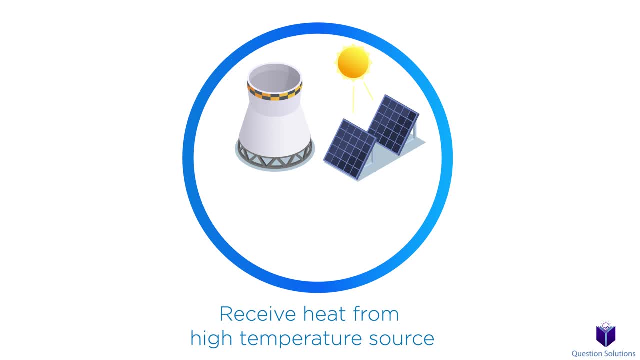 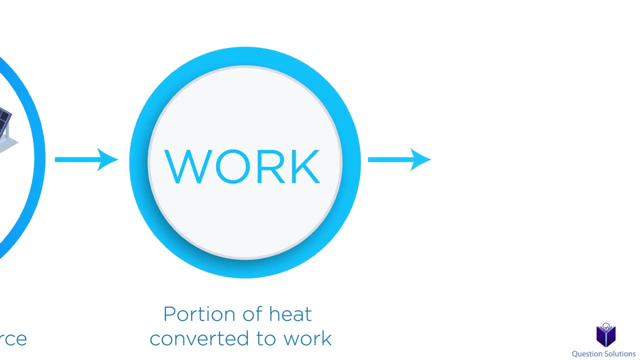 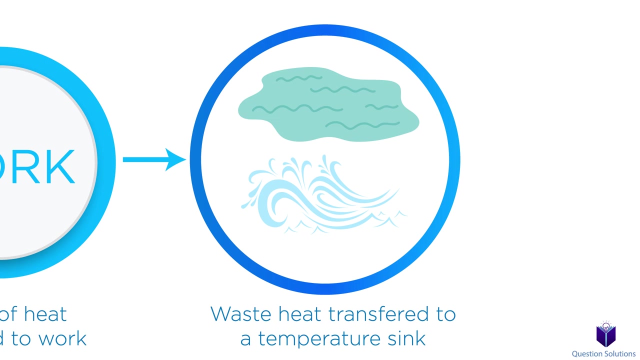 So from a nuclear reactor, solar energy, hot oil, things like that, They convert a portion of this heat into work. The remaining waste heat is transferred to a temperature sink. That could be the atmosphere, a water source like a lake, anything that can safely absorb the temperature and 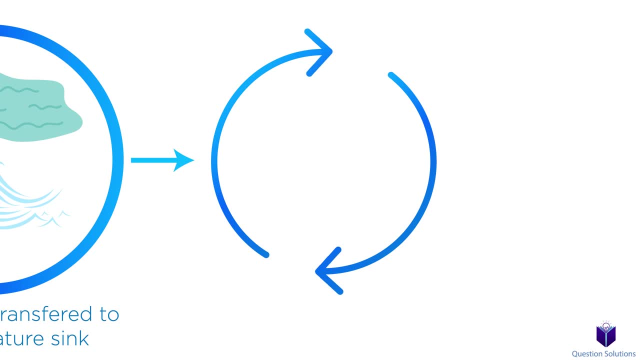 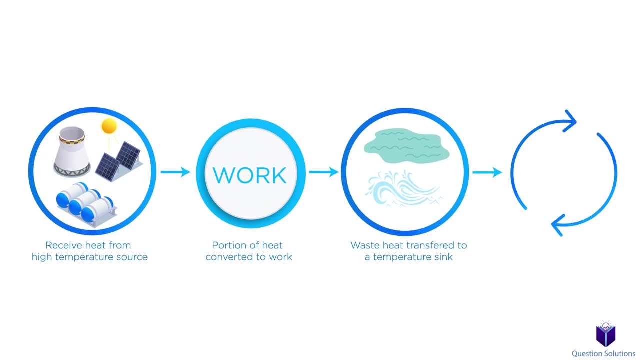 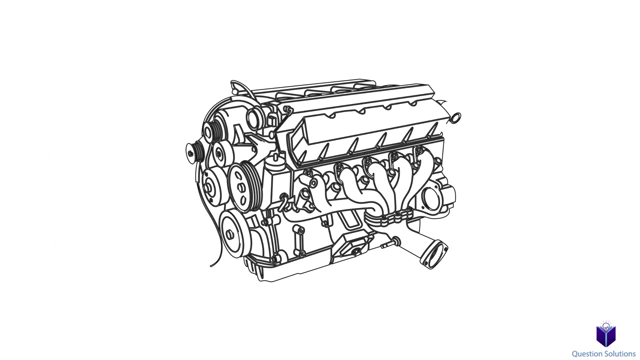 dissipate it. Lastly, they operate on a cycle. You might also hear a term called the working fluid. That's referred to the fluid that carries heat during a heat engine cycle. Now, you probably thought about a car engine when we were talking about these characteristics. 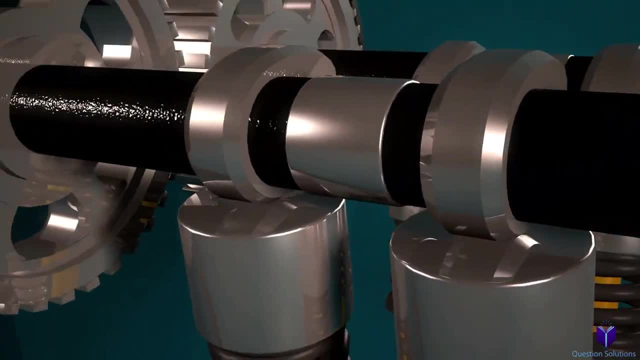 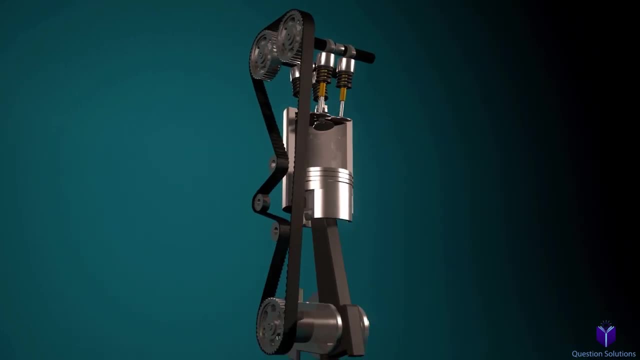 You guessed it right: this efficiency runs on the basis of heat And, yes, a car engine does fall into the broad category of a heat engine, But it actually operates in a mechanical cycle, not a thermodynamic cycle. What we're interested in, for now at least, 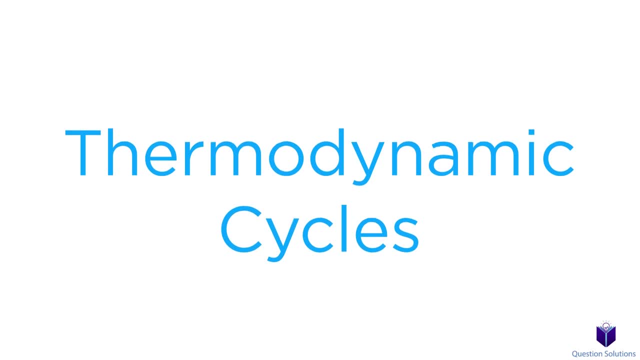 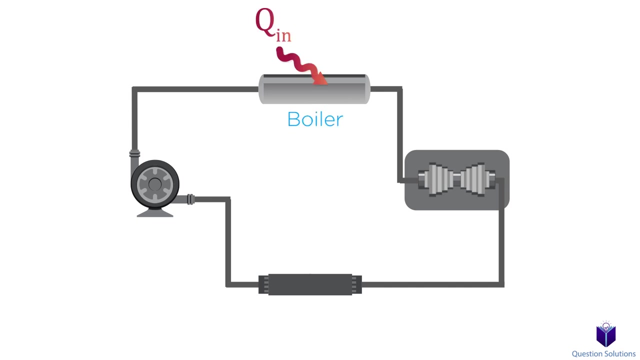 are thermodynamic cycles. We will talk about mechanical cycles in a future video. A great example of a thermodynamic cycle is the steam power plant would look like this: Here some external energy source is used to heat the water into steam inside a boiler, In other words heat input. The steam then enters the turbine, it spins and then we. 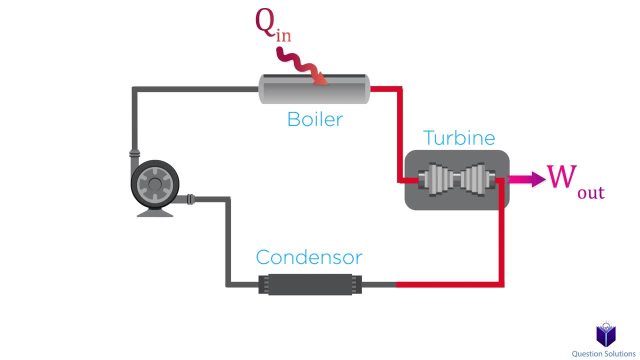 get work output From there. the steam enters a condenser and the heat is dissipated into an energy sink. That could be to the atmosphere or a river. Here there is heat output. The liquid is then pulled through a pump and goes back into the boiler to be heated up again and turned into steam. 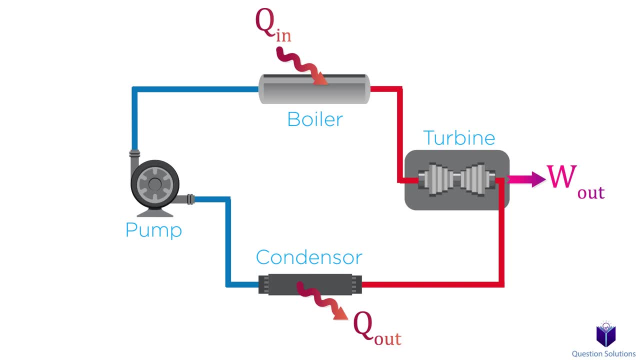 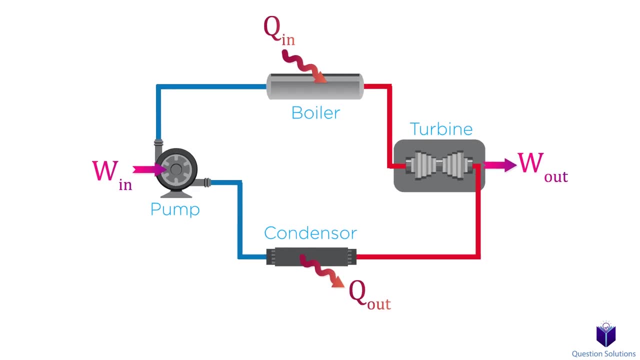 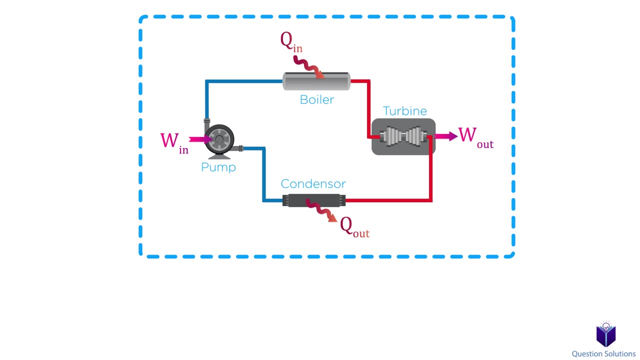 Keep in mind that work must be supplied to the pump for it to work, so there is work input here. This whole process is a thermodynamic cycle and we can take this whole process to be our system. In simple terms, we added heat to the system and got work output, and that's a heat engine, The network of this. 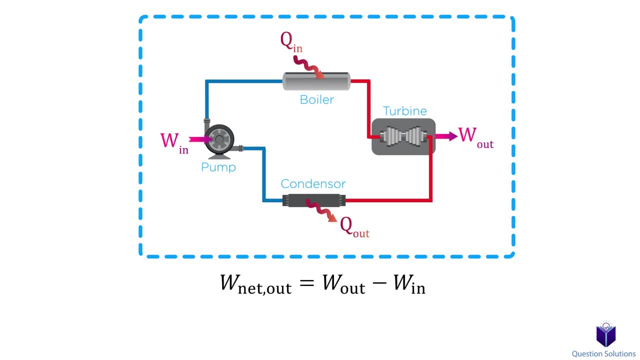 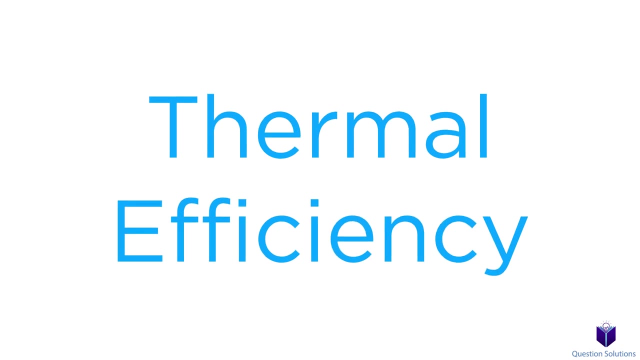 power plant can be found by subtracting work input from the work output. Another way to figure out the network is to subtract heat output from the heat input. since this is a closed system, An important factor to consider is the thermal efficiency of a cycle. Thermal efficiency tells us how great a heat 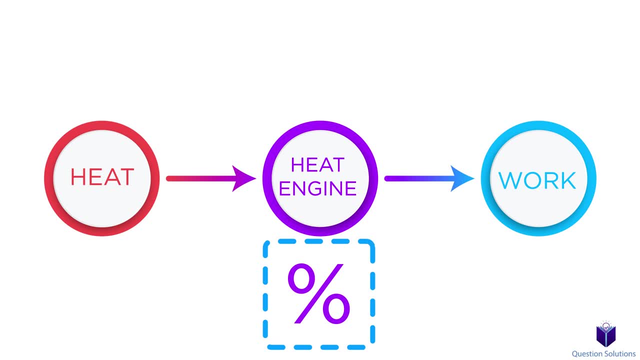 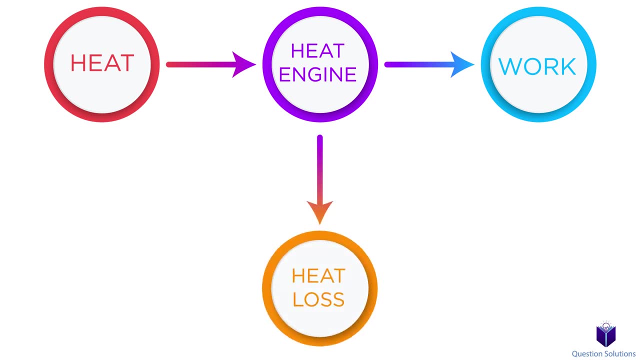 engine does and how much heat the system produces. The thermal efficiency of a cycle is the thermal efficiency of a cycle. The thermal efficiency of a cycle tells us how great a heat engine does at converting heat to work. Needless to say, the heat output is always less than the amount of heat input. In simple terms, 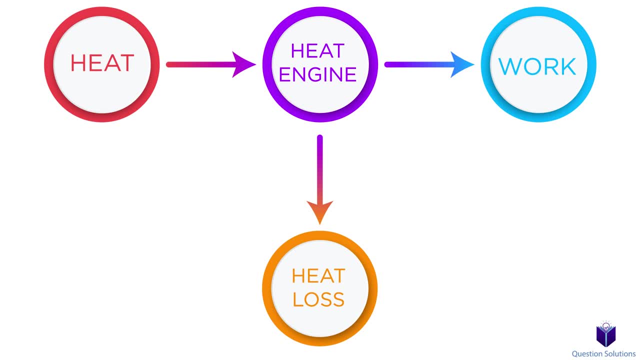 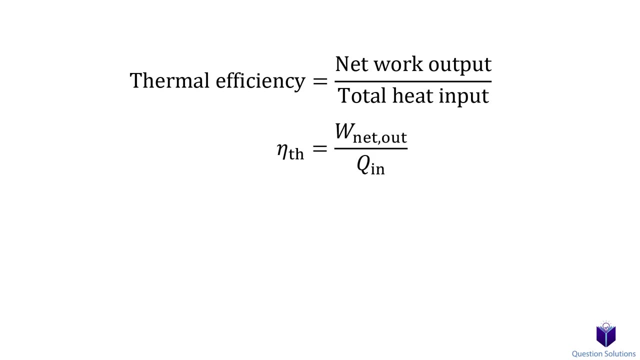 only some of the heat transferred is converted to work. If we want to figure out the efficiency then we need to divide the network output by the total heat input and that would give us the thermal efficiency. Remember from before that network can be found by subtracting heat output from the heat input. 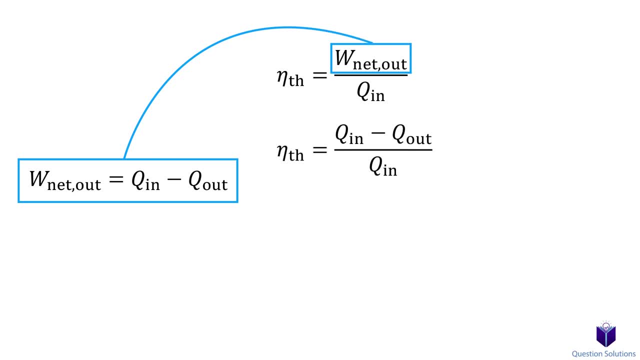 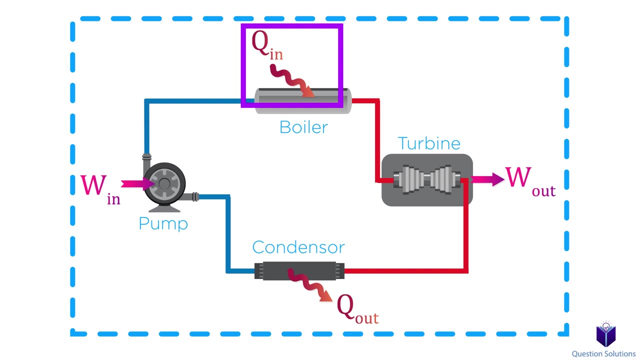 So if we plug that into the equation and do a bit of tidying up, we can write the efficiency like this: Let's go back to our steam power plant example. This was our whole system and we said that we have heat input here and heat output here, Instead of thinking of singular heat inputs and outputs. 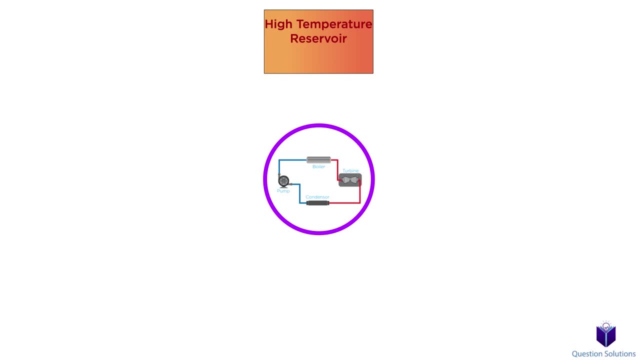 we can think of it as a high temperature reservoir here and a low temperature reservoir down below. We will label the high temperature reservoir as TH and low temperature reservoir as TL. Now the high temperature reservoir transfers some heat into our cycle, The magnitude of heat that's. 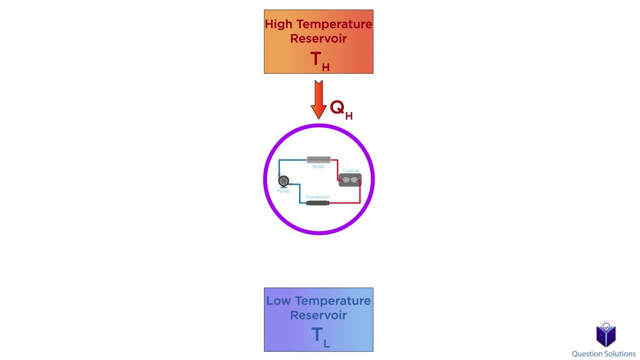 transferred. we're going to label that QH. At the other side, some waste heat is transferred from the cycle into the low temperature reservoir. The magnitude of that transfer, we will label QL. So in simple terms, QH gives us the magnitude of heat transfer between the high temperature reservoir and the cycle. 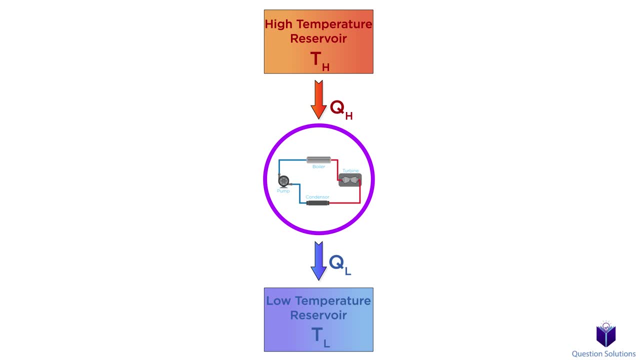 and QL gives us the magnitude of heat transfer between the low temperature reservoir and the cycle. Keep in mind: QH and QL are magnitudes, which means they will always have positive values. With that, we can write our efficiency equations using these new terms. So heat input is just the 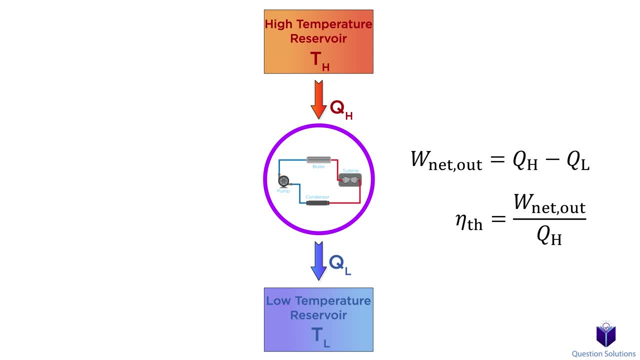 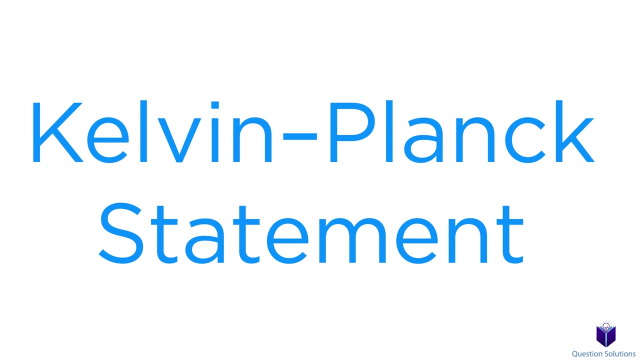 magnitude of heat transfer between the cycle and the high temperature reservoir, and heat output is the magnitude of heat transfer between the cycle and the low temperature reservoir. There is one more thing that needs to be mentioned, and it's called the Kelvin-Planck statement. It says that it's impossible for a device that operates on a cycle 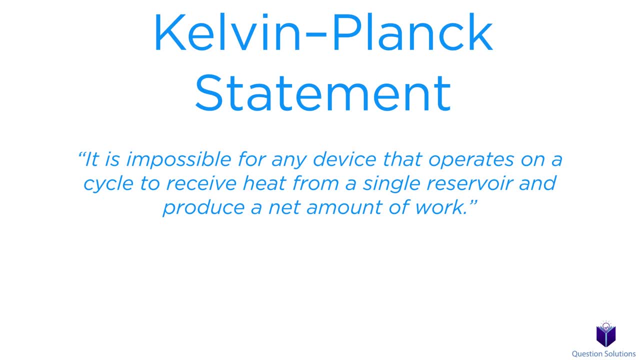 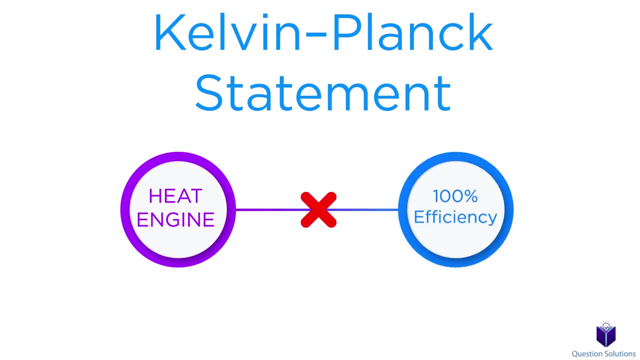 to receive heat from a single reservoir and produce a net amount of work. What this means is that- no heat engine can ever have a thermal efficiency of 100%. In other words, we can never have an engine that converts all of the heat into an equal amount of work When we dive deep into 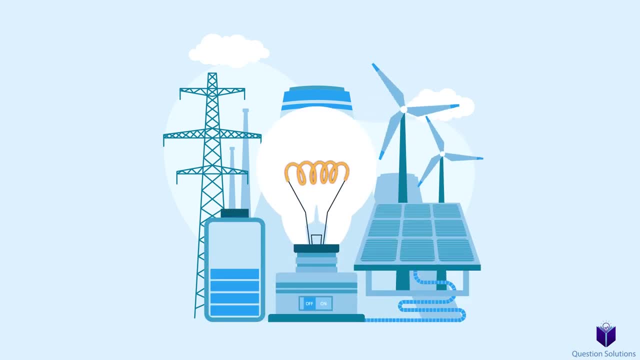 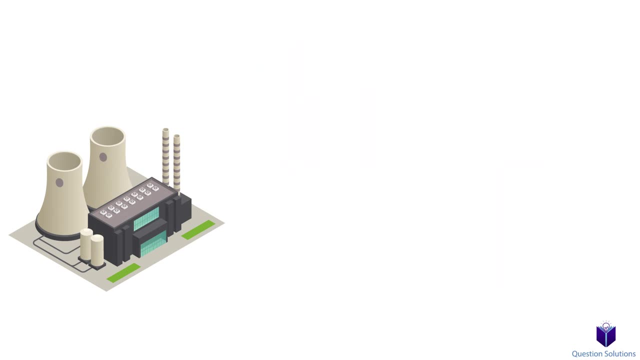 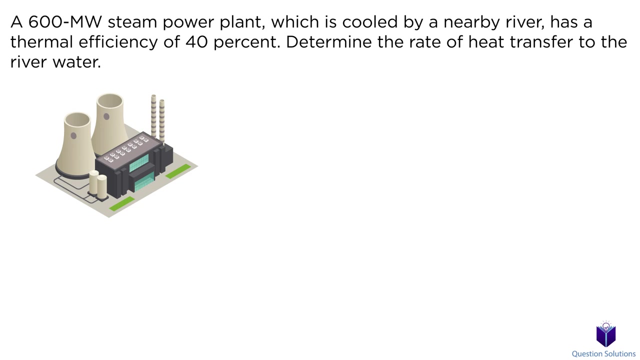 maximum thermal efficiency. in a future video we will talk about why this is true. Now let's go through some examples to understand what we talked about. Let's take a look at this question where we have a steam power plant, It's cooled by a nearby river and we need to figure out the rate of heat. 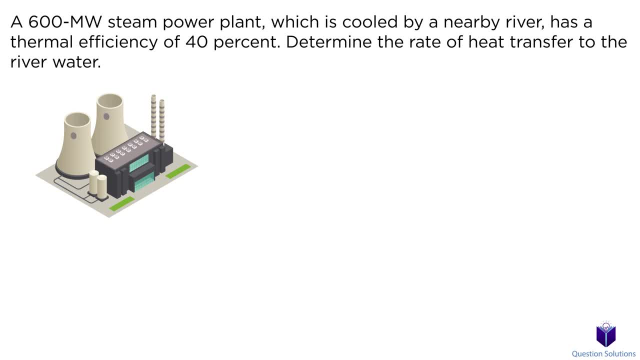 transfer to the river. We will start off by writing down what we know. The network output is 600 megawatts. Remember, this is rate form, in other words power per second, because one watt is one joule per second, so there's a dot on top. The thermal efficiency is 40 percent. 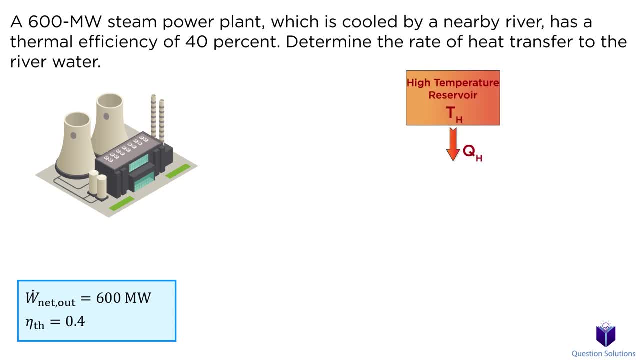 Let's draw a comment diagram. So we have a high temperature reservoir here and the cycle, and then we have the low temperature reservoir here, which in this case is a river. What we need to find is the magnitude of heat transfer between the cycle and the river QL. Using the givens, we can first figure out QH. 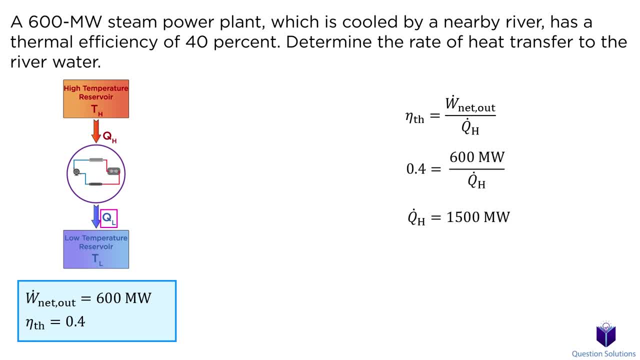 Let's plug in what we know. Now we can solve for QH, which is the magnitude of heat transfer to the power plant. Next, we just need to use our network equation to figure out the rate of heat transfer to the river. Let's plug in our values and solve for QL. This tells us that 900 megawatts. 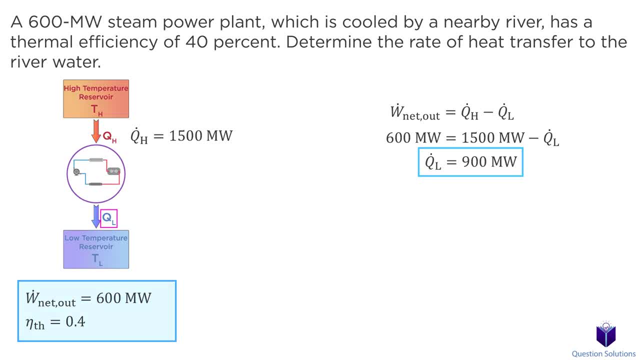 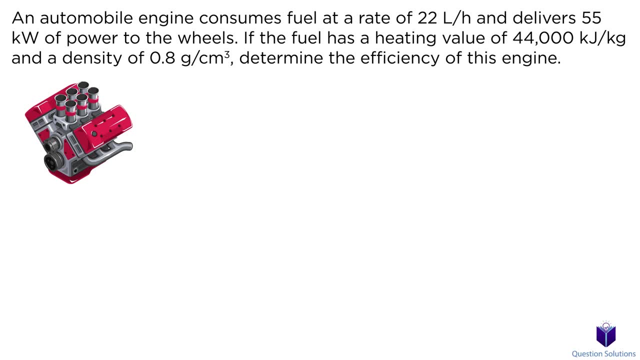 of heat was transferred to the river. Let's take a look at this question where we need to figure out the efficiency of an automobile engine. We can start by writing down what we know. The fuel consumption rate of the engine is 22 liters per hour and it delivers 55 kilowatts of power to the wheels. 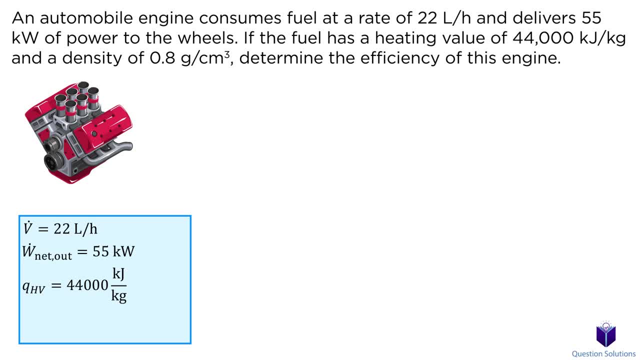 The fuel has a heating value of 44,000 kilojoules per kilogram and a density of 0.8 grams per cubic meter, which is the same as 0.8 kilograms per liter. We know the equation for thermal efficiency. 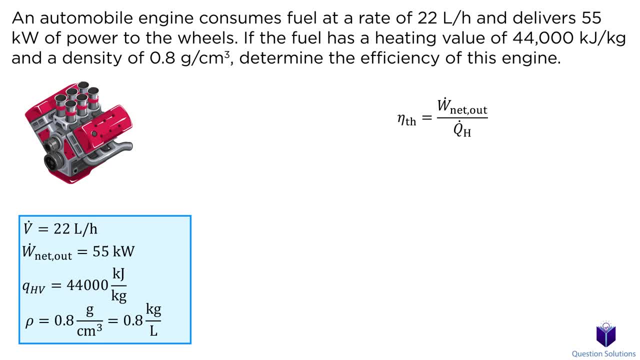 Let's write it down: We have the net power, but we don't have the rate of heat supply. So let's figure that out first. The rate of heat can be found by multiplying mass flow by the heating value of a substance. We can write that like this: We have the heating value, but we don't have the mass flow. 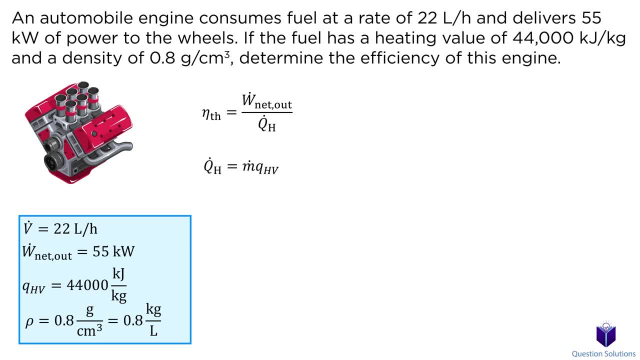 so let's go and figure that out. Mass flow is equal to density multiplied by volume flow. If this is unfamiliar to you, please watch the video on mass flow and volume flow. Let's plug in our givens. Solving tells us that 17.6 kilograms of fuel is consumed every hour. Now we just need to plug this. 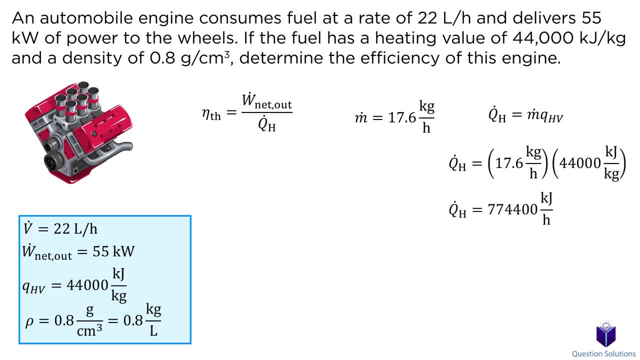 into our heat rate equation. Solving gives us the heat supply rate to the car and if we divide this by 3600 seconds, we can write it in kilowatts. The last step is to plug this value into our thermal efficiency equation. 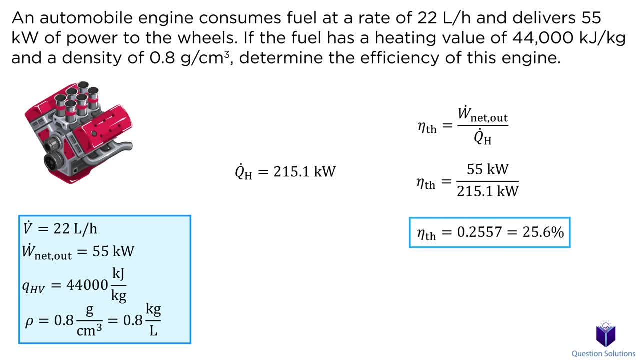 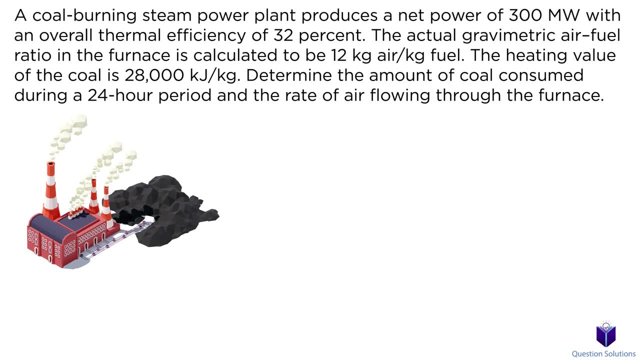 This tells us that the engine is 25 percent efficient. Let's take a look at this problem where we have a steam power plant. We need to find the amount of coal consumed by the plant in a 24-hour period and the rate of air flow through the furnace. 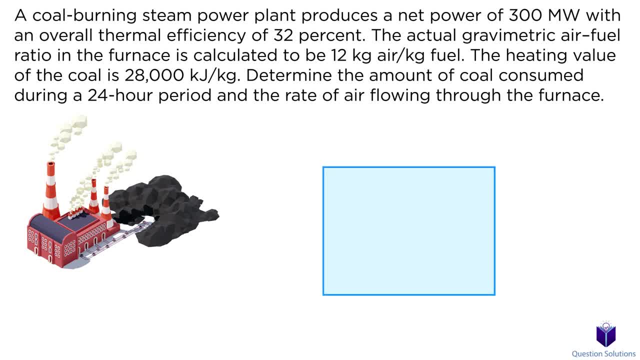 Let's start by writing down what we know. The net power the power plant produces is 300 megawatts. The thermal efficiency is 32 percent. We're given the air-to-fuel ratio in the furnace and it's 12 kilograms of air. 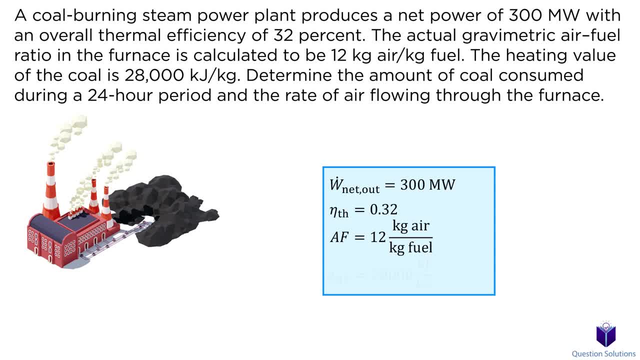 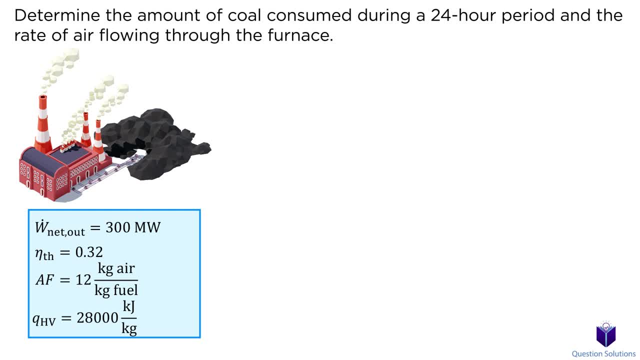 per kilogram of fuel. Lastly, the heating value of the coal is 28,000 kilojoules per kilogram. We can figure out the rate of heat input using the efficiency equation, Since the question is asking for the amount of coal consumed in a 24-hour period.